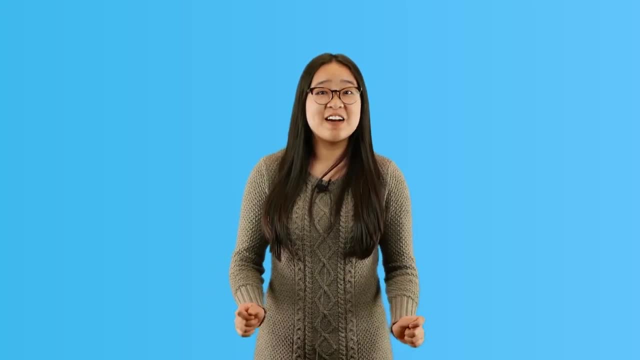 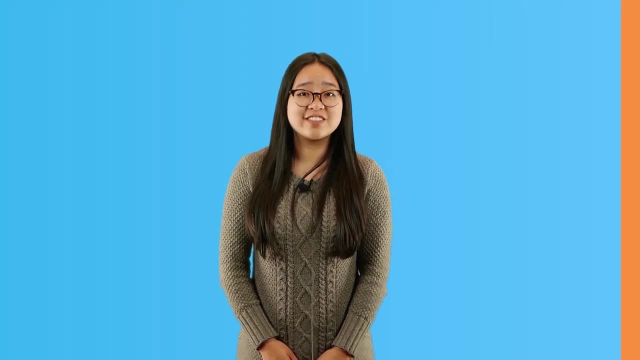 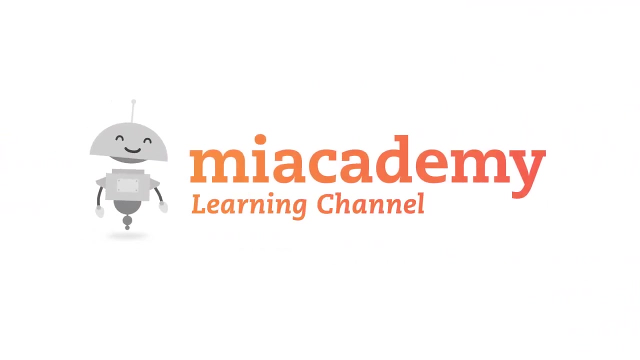 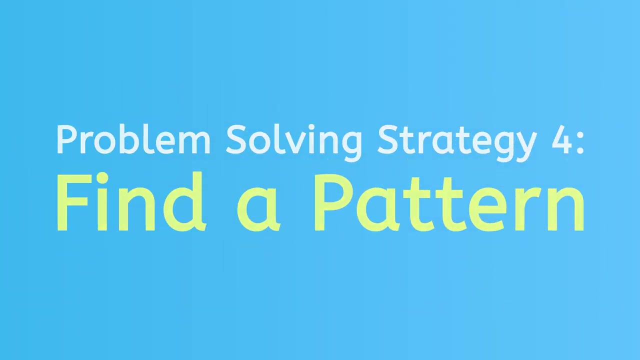 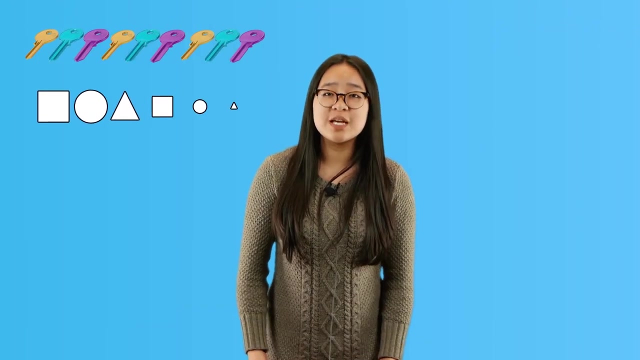 Hello and welcome to problem solving strategy number four: find a pattern. In this video, you'll learn how to look for patterns in a word: problem to help you come to a solution. Patterns are found everywhere in our world. Patterns can be repeated items, shapes, colors. 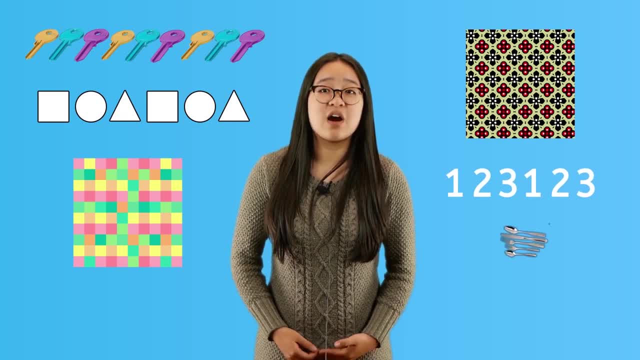 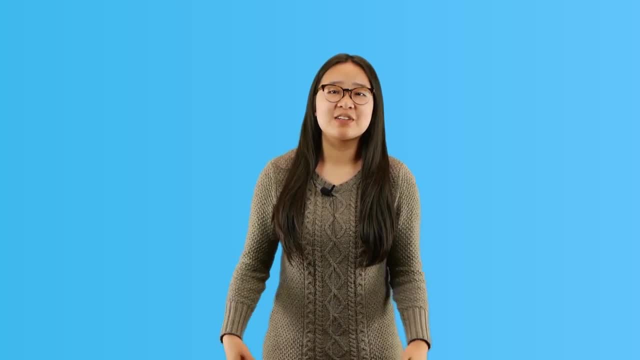 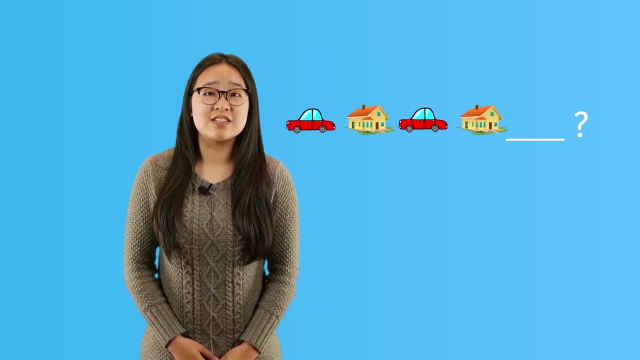 images or numbers. Sometimes a set of these are repeated to create a pattern. Some math problems can be solved by finding a pattern. Sometimes the patterns are obvious, such as with this visual pattern. This problem asks what comes next in the pattern. Remember. 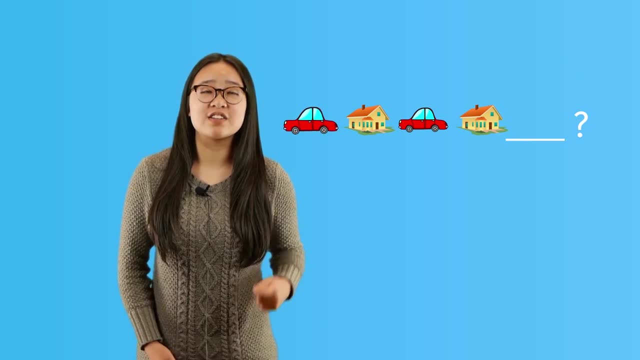 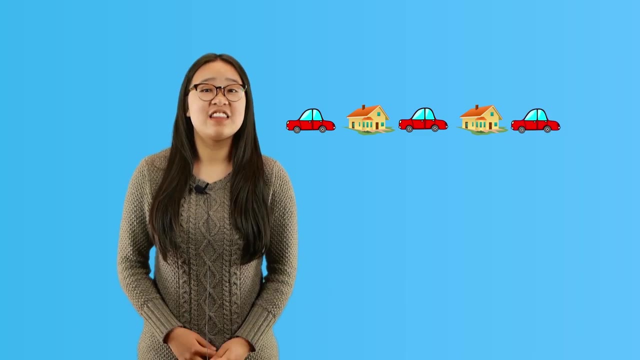 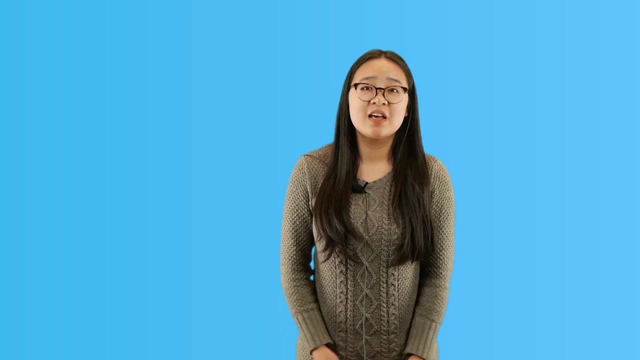 a pattern means repeated images. In this case, there's a car, a house, a car, a house. What comes next? Right, a car. That was fairly easy to find. Sometimes the pattern is not so clear, such as in this word: problem A. 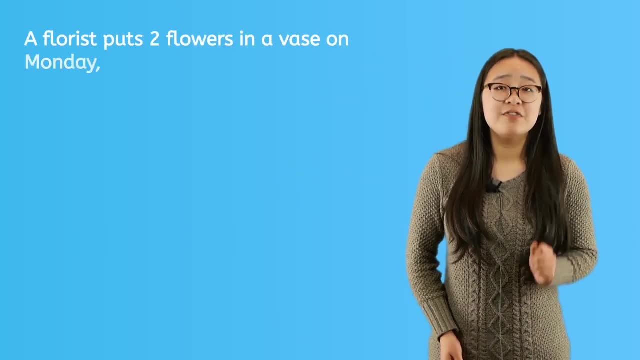 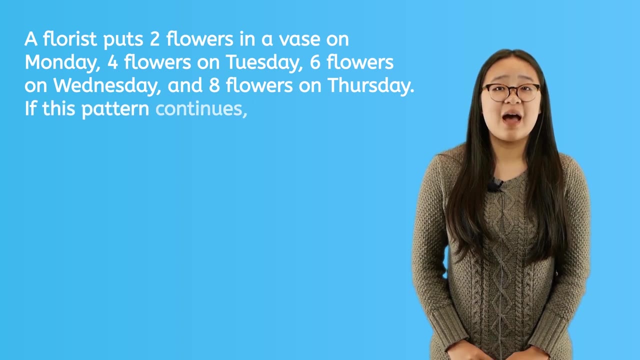 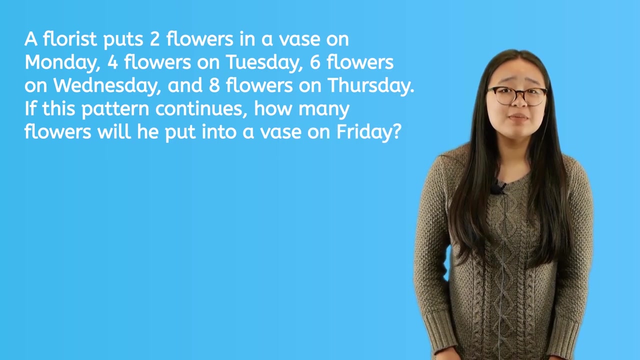 florist puts two flowers in a vase on Monday, four flowers on Tuesday, six flowers on Wednesday and eight flowers on Thursday. If this pattern continues, how many flowers will he put into a vase? What's��는? and eight flowers. This is also difficult because we can't come up with a pattern. 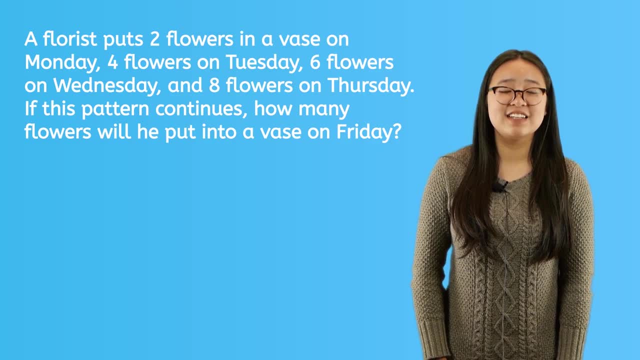 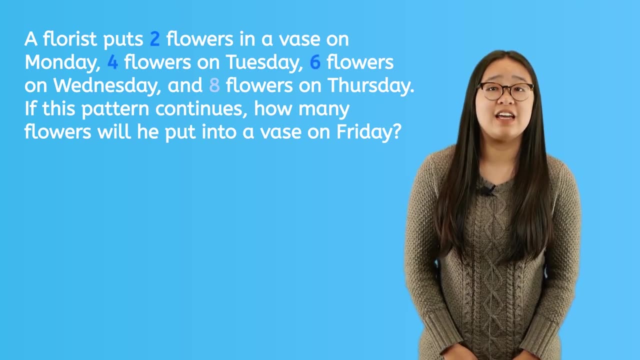 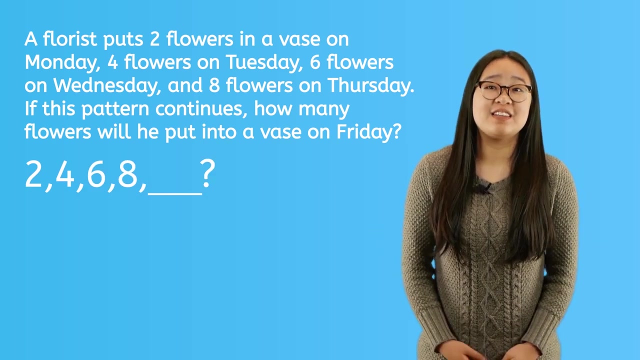 Let's find out what this flower wheel looks like. or put two flowers into the oval and put up a flower and a star. It looks like this. It looks like these real flowers. The florist does not understand this and gives her the pattern a hard time human. 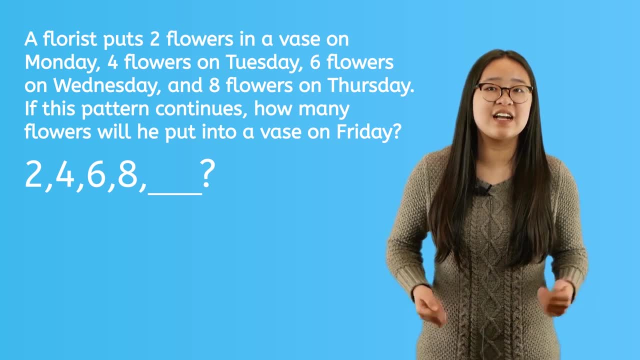 8the florist adds two more flowers to the vase, going from the best to the worst. As soon as the flowerdaily appears, the florist starts to evaluate each flower in the world than he added the day before. The pattern is counting by twos. 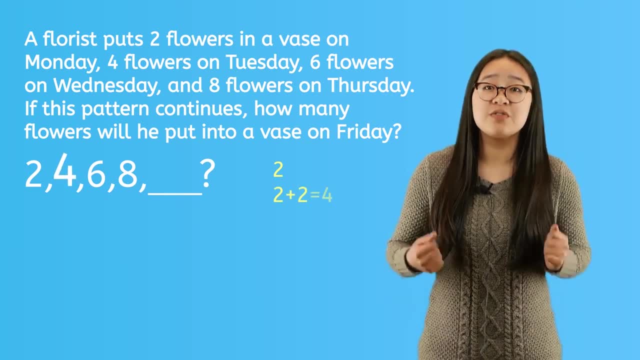 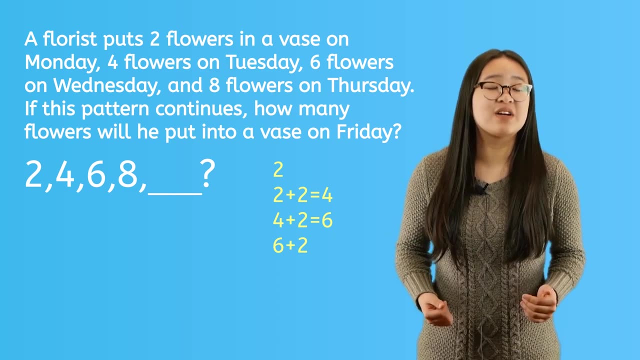 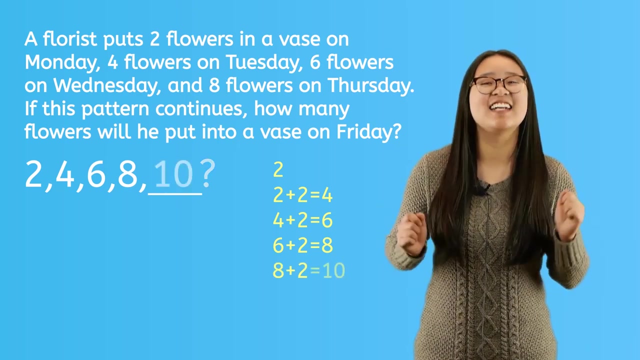 So 2 plus 2 gave the florist 4.. 4 plus 2 gave the florist 6.. 6 plus 2 gave the florist 8 flowers. That means we need to add 2 to 8 to give us 10.. 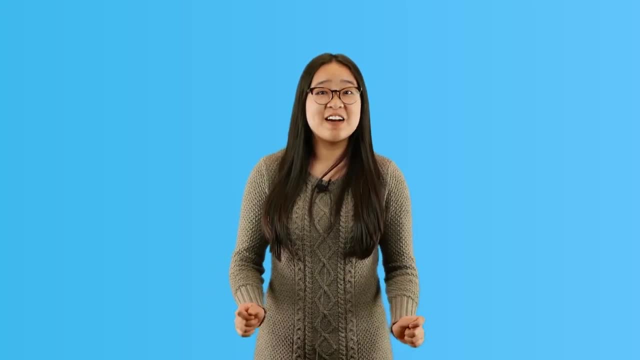 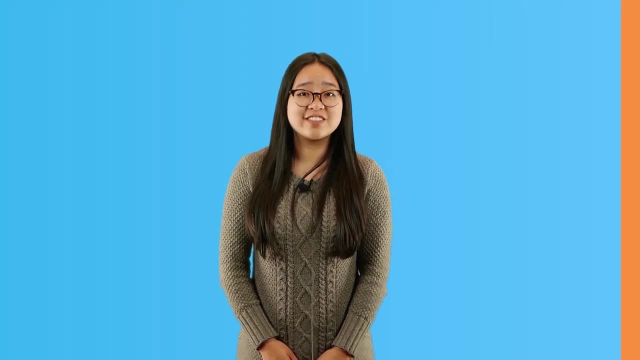 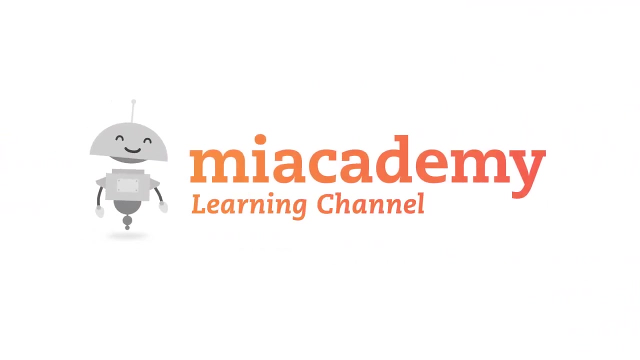 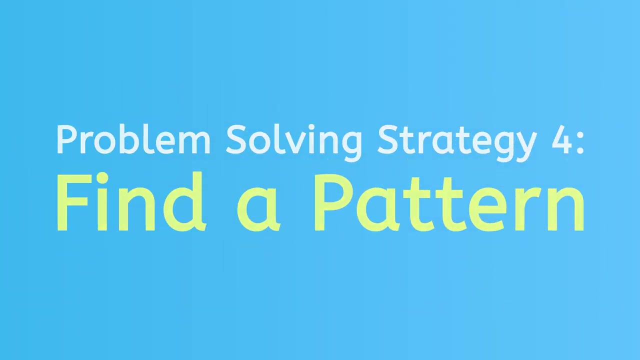 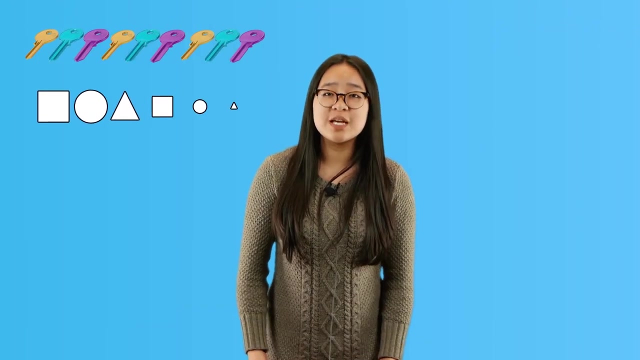 Hello and welcome to problem solving strategy number four: find a pattern. In this video, you'll learn how to look for patterns in a word: problem to help you come to a solution. Patterns are found everywhere in our world. Patterns can be repeated items, shapes, colors. 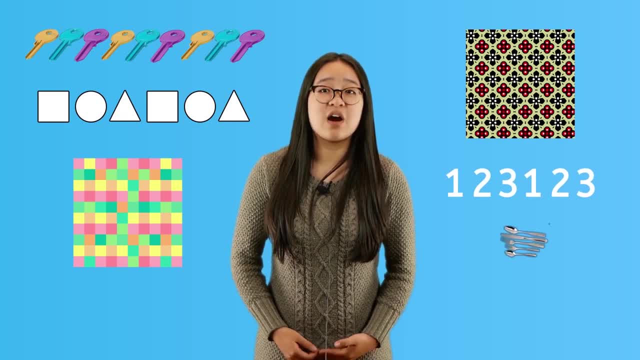 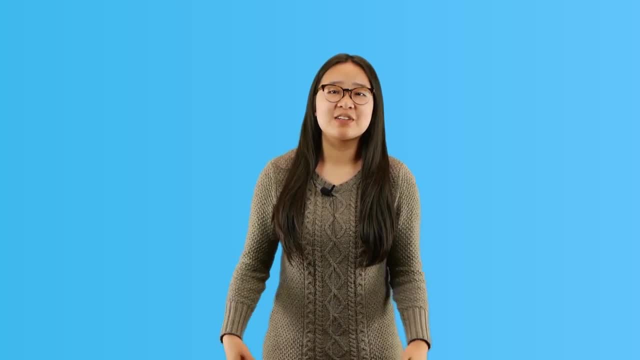 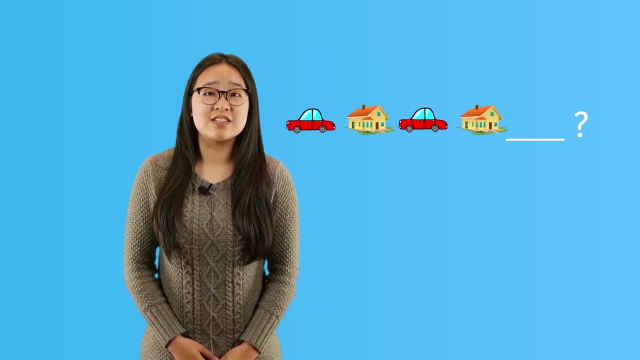 images or numbers. Sometimes a set of these are repeated to create a pattern. Some math problems can be solved by finding a pattern. Sometimes the patterns are obvious, such as with this visual pattern. This problem asks what comes next in the pattern. Remember. 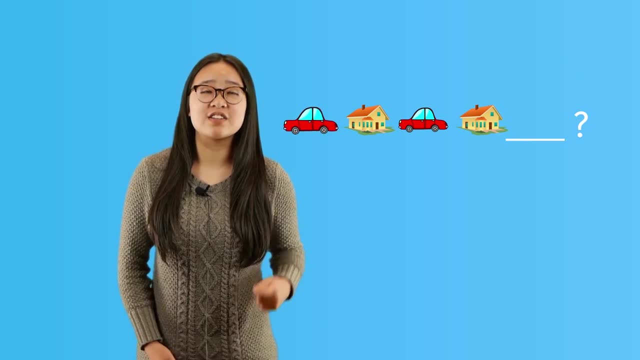 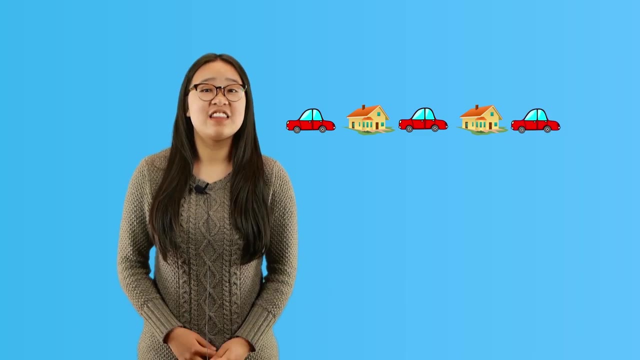 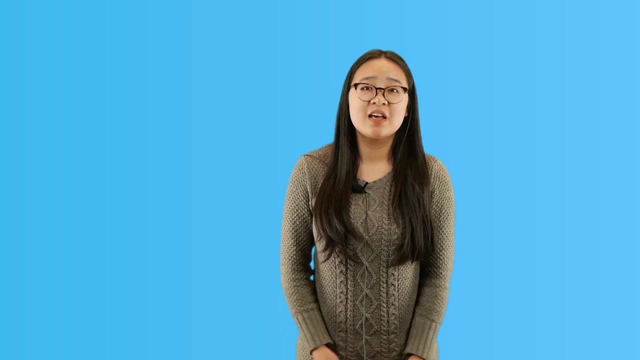 a pattern means repeated images. In this case, there's a car, a house, a car, a house. What comes next? Right, a car. That was fairly easy to find. Sometimes the pattern is not so clear, such as in this word: problem A. 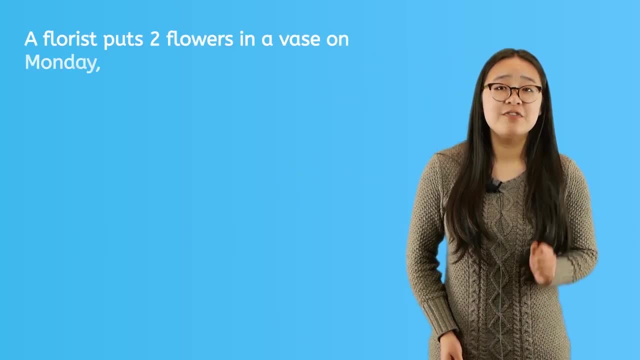 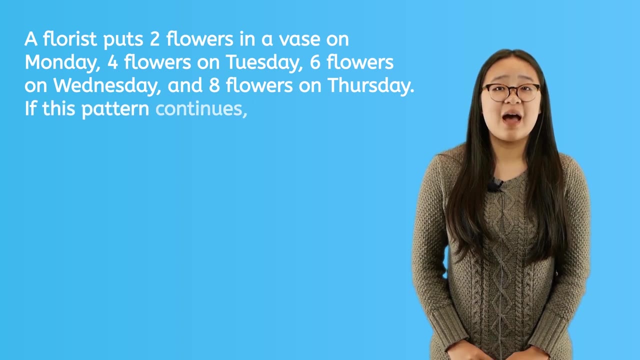 florist puts two flowers in a vase on Monday, four flowers on Tuesday, six flowers on Wednesday and eight flowers on Thursday. If this pattern continues, how many flowers will he put into a vase? The answer is obvious. Another platforms has not arrived yet, so find it on Thursday. 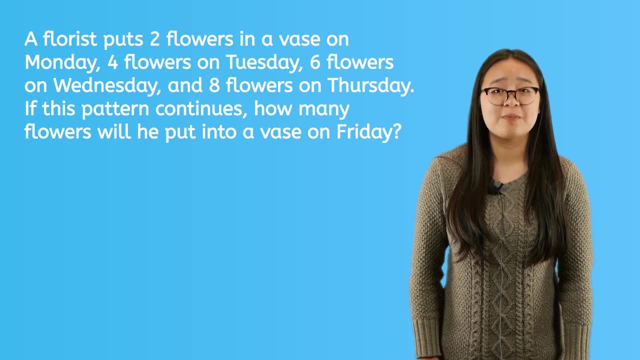 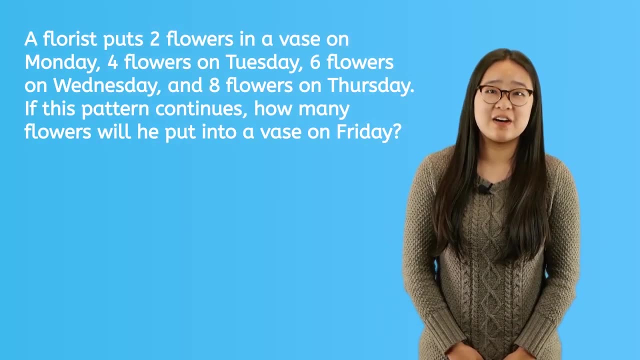 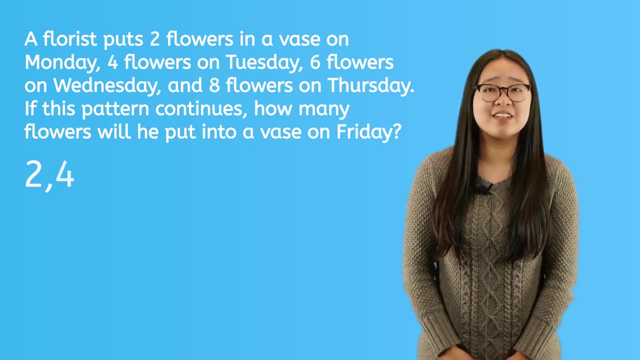 This problem is tricky because there aren't any pictures to help us out. That's because it's a numeric or number pattern. Let's find the patternHere's the pattern so far: 2,4,6,8.. What comes next to complete the pattern? 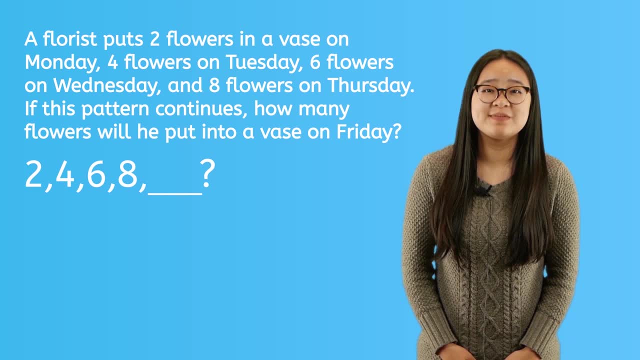 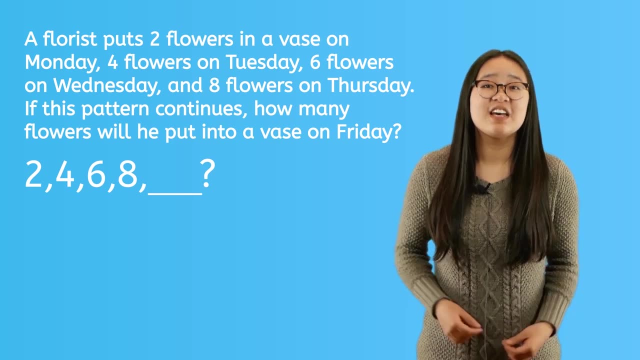 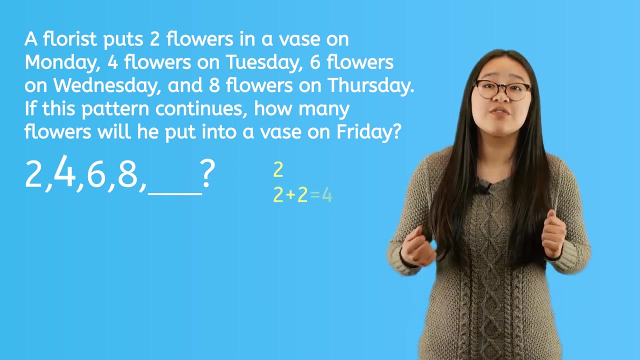 Well, what is really happening in this pattern? Each day the florist adds two more flowers to the vase than he added the day before. The pattern is counting by twos. So two plus two gave the florist four. Four plus two gave the florist six. 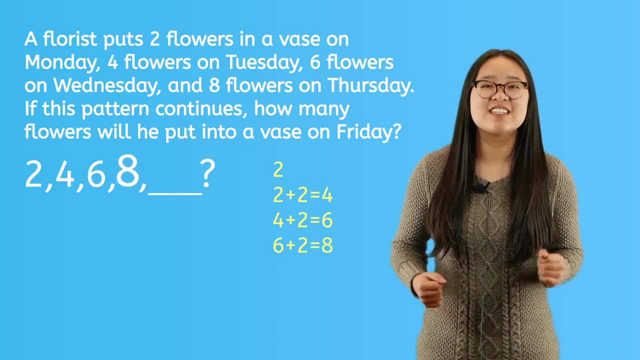 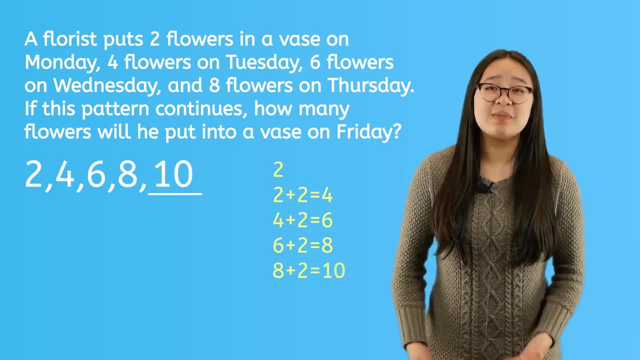 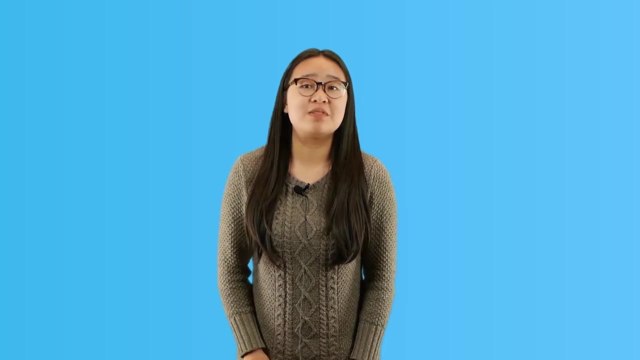 Six plus two gave the florist eight flowers. That means we need to add two to eight to give us 10.. Yes, the pattern is two, four, six, eight, 10.. Look for patterns in your world and in word problems to help you solve them.